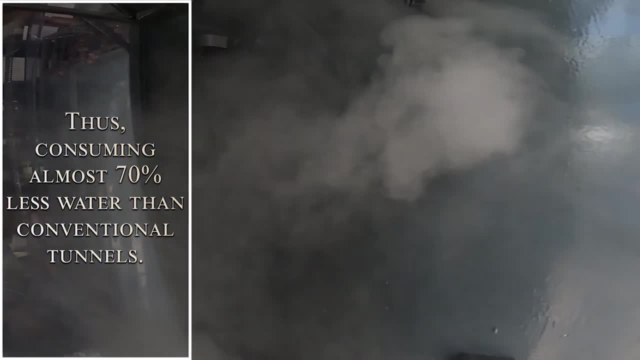 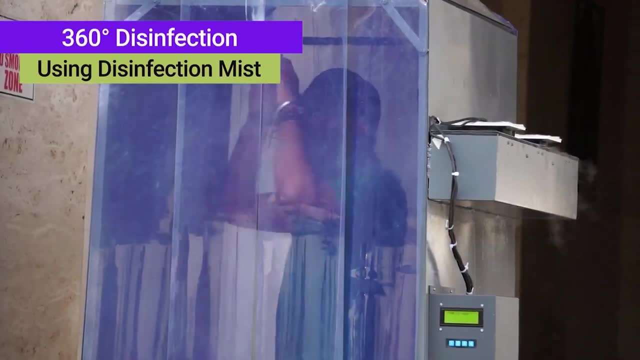 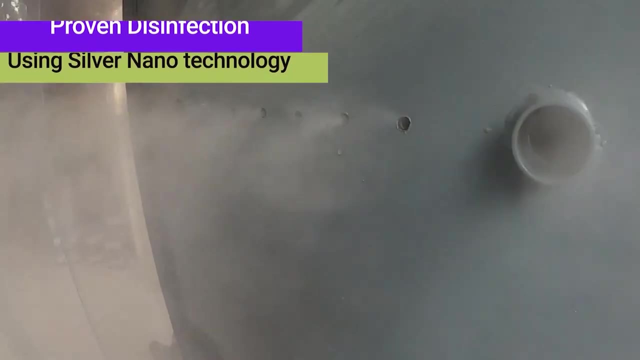 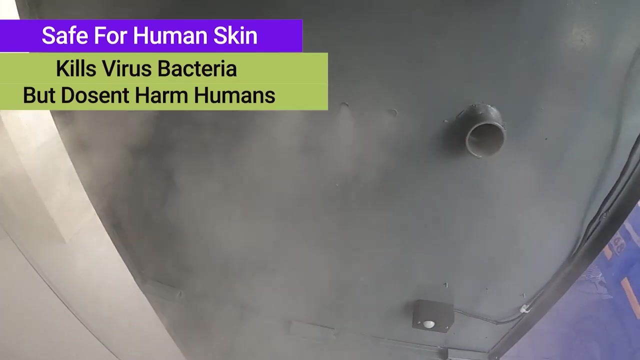 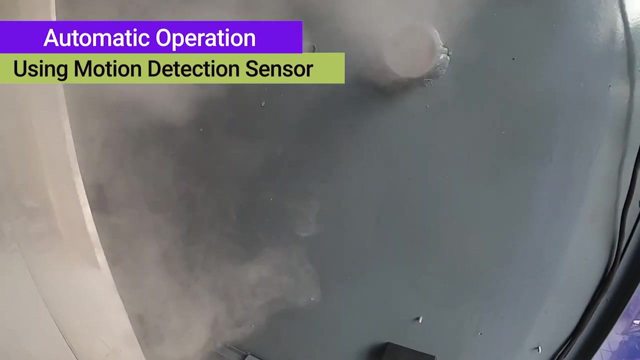 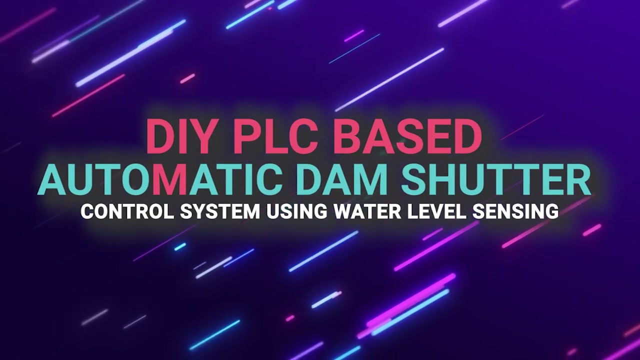 thus consuming almost 70% less water than conventional tunnels. In addition, these tunnels use a lot of water and also a lot of dust. This means that the water can easily be washed away. DIY PLC-Based Automatic Dam Shutter Control System Using Water Level Control System. 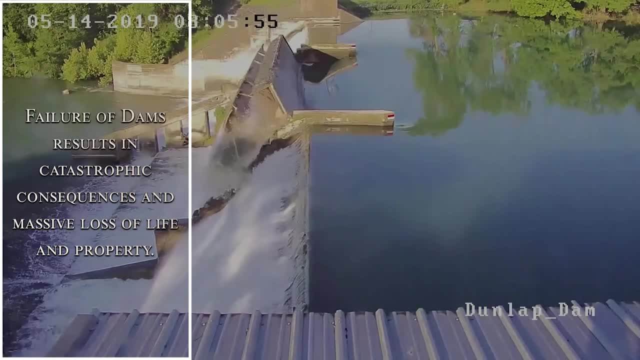 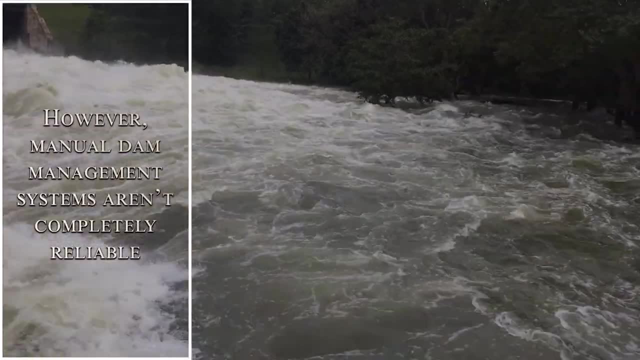 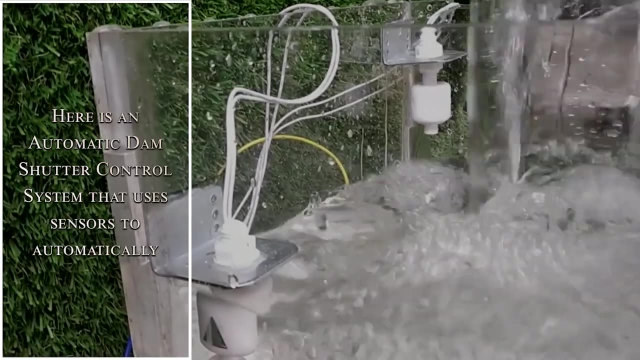 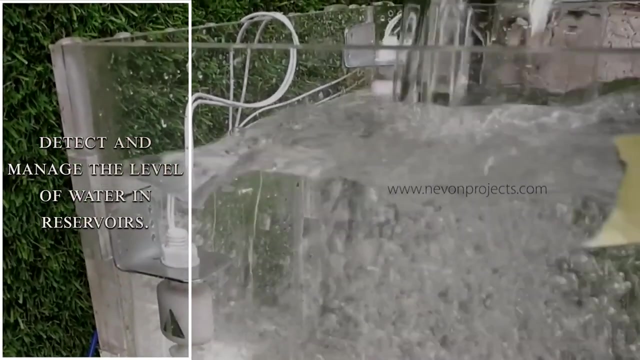 DIY PLC-Based Automatic Dam Shutter Control System. Using Water Level Control System. Using Water Level Sensing. Using Water Level Sensing- Community in EVER. Professional Damp Management System. Use Water Level Sensing- Rerical sensing. failure of dams results in catastrophic consequences and massive loss. 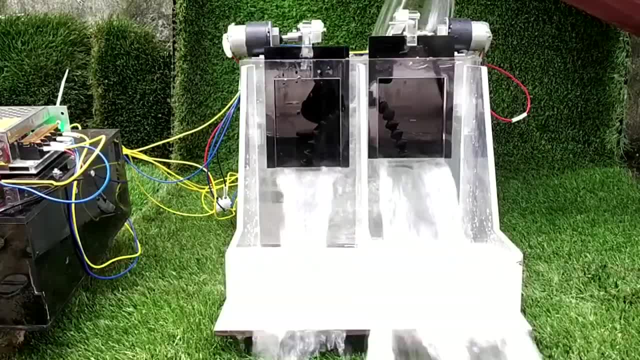 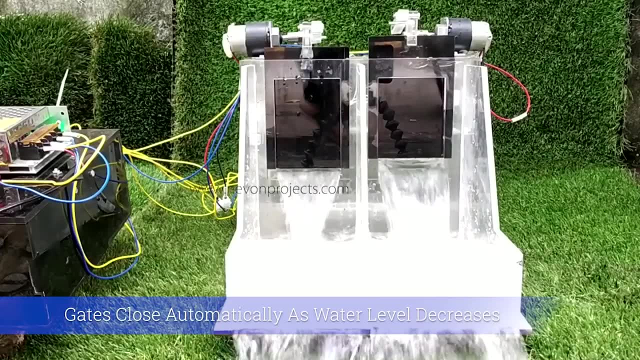 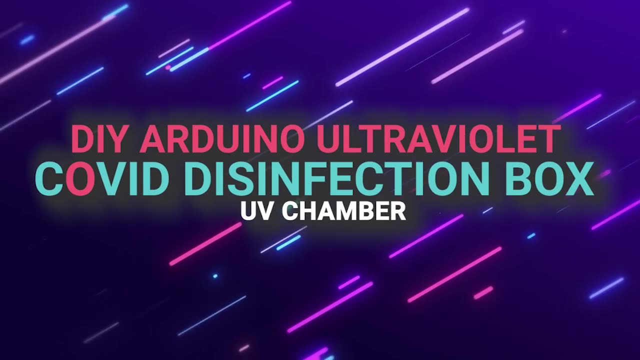 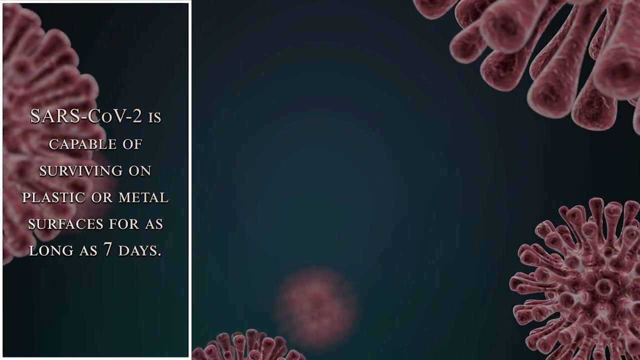 of life and property. However, manual dam management systems aren't completely reliable, So here is an Automatic Dam Shutter Control System that uses sensors to automatically DIY Arduino Ultra Voilet Covid Disinfection Box. SARS-CoV-2 is capable of surviving on plastic or metal surfaces for as long as 7 days. 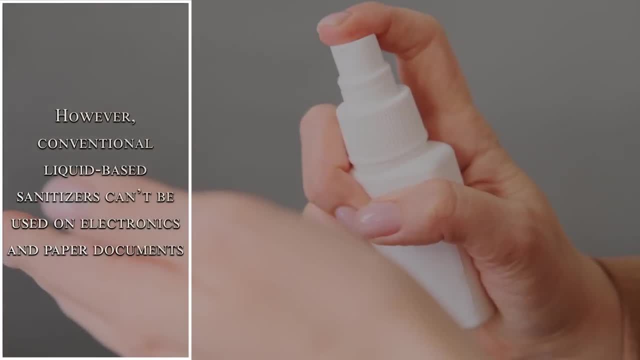 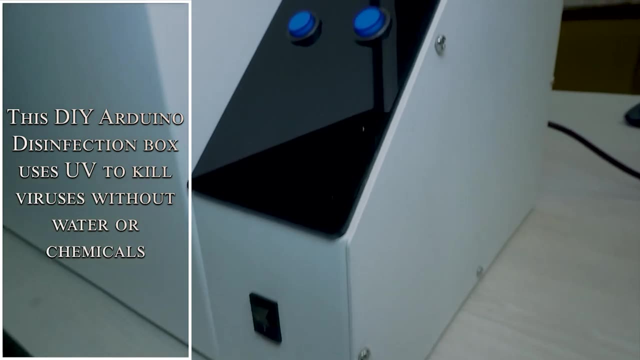 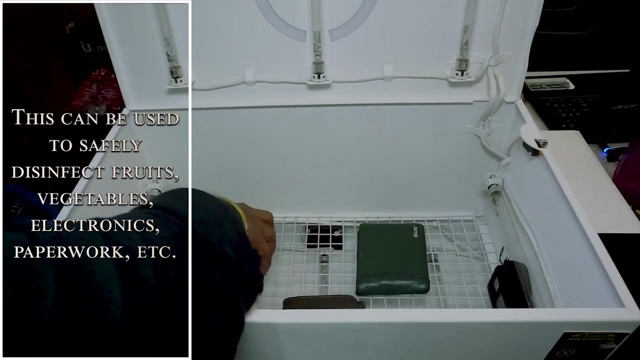 However, conventional liquid-based sanitizers can't be used on electronics and paper documents, So this DIY Arduino Disinfection Box uses UV to kill viruses without water or chemicals. This can be used to safely disinfect fruits, vegetables, electronics, paperwork, etc. 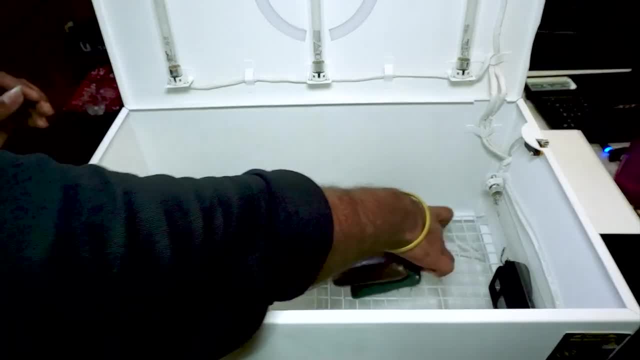 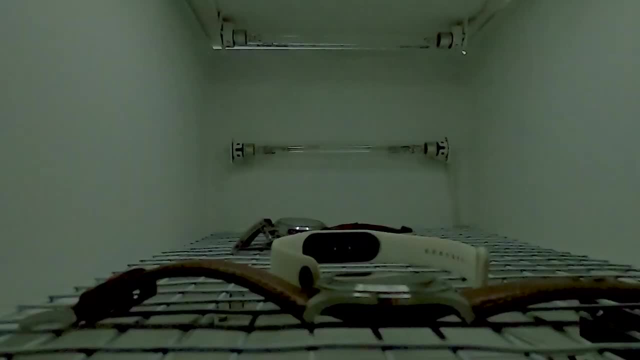 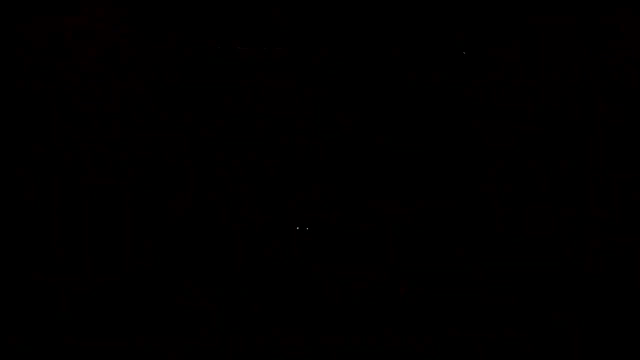 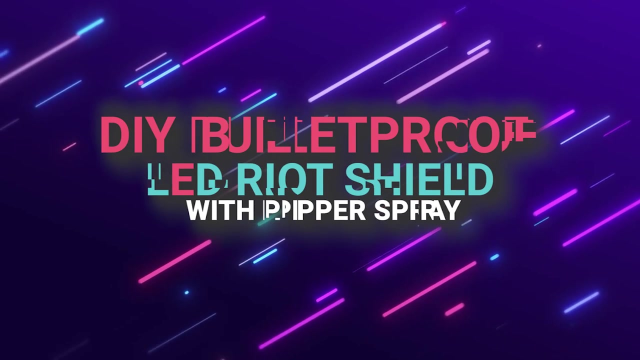 DIY Bulletproof LED Ride Shield with Paper Spray. When ride is free, the LED will be lit. The LED will be lit when the ride is free. The LED will be lit when the ride is free. The LED will be lit when the ride is free. 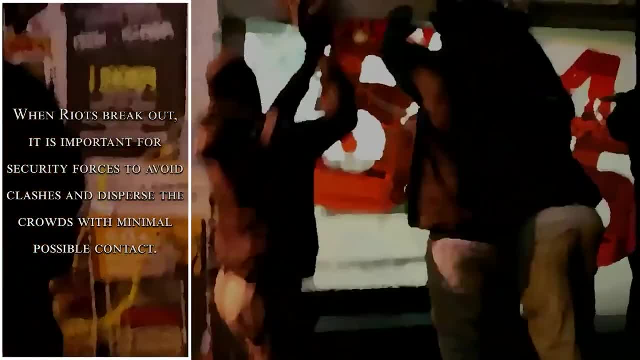 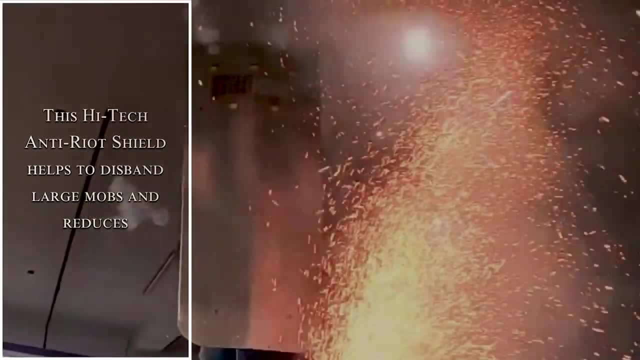 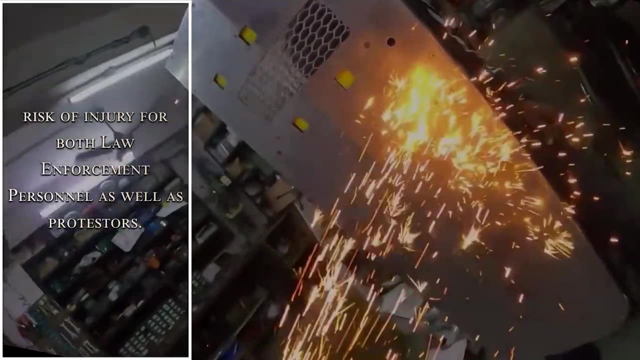 To take out. it is important for security forces to avoid clashes and disperse the crowds with minimal possible contact, So this high-tech anti-ride shield helps to disband large mobs and reduces risk of injury for both law enforcement personnel as well as protesters. 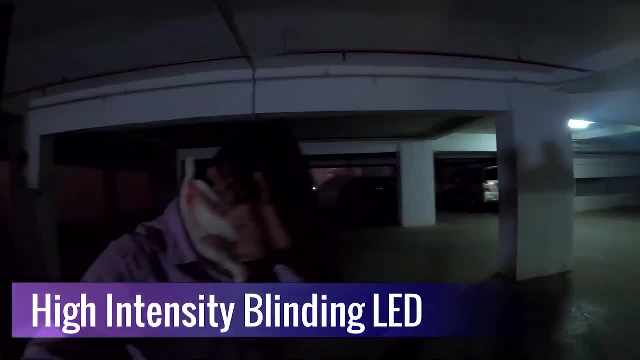 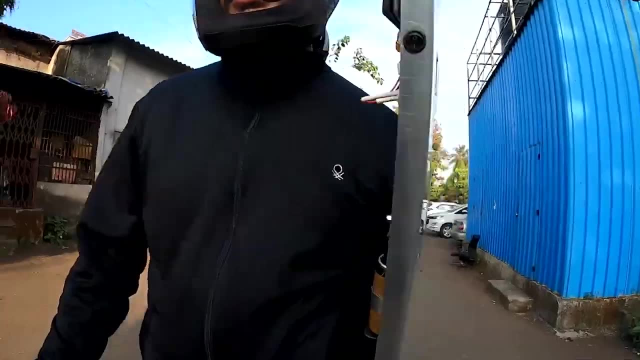 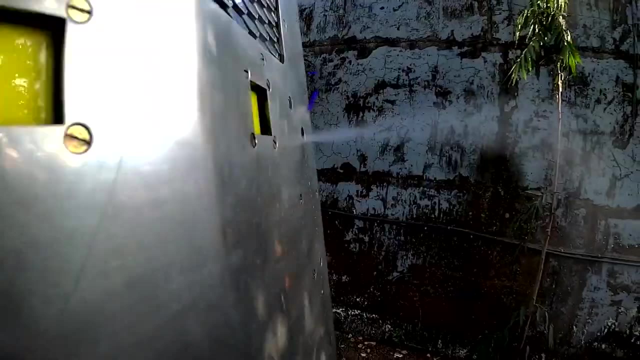 To take out. it is important for security forces to avoid clashes and disperse the crowds with minimal possible contact To take out. it is important for security forces to avoid clashes and disperse the crowds with minimal possible contact To Mit aujourd với loétgeput. 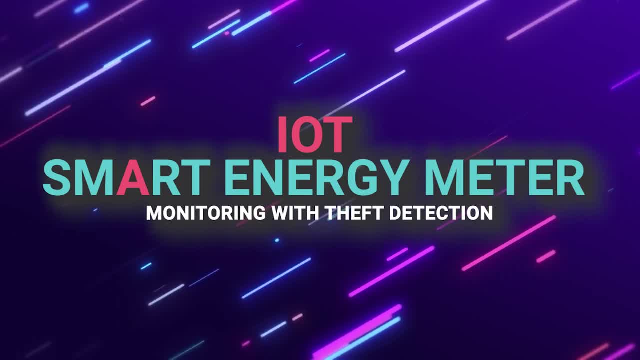 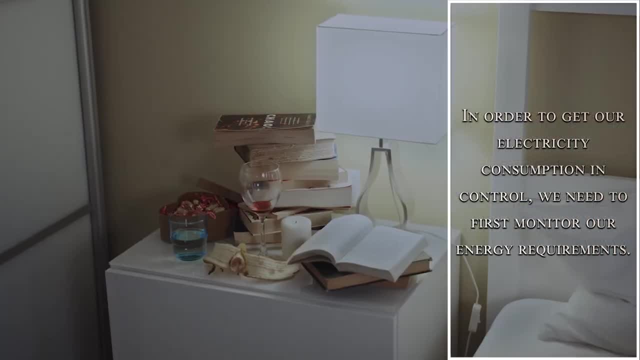 IoT Smart Energy Meter Monitoring with Theft Detector: Ulılaşa penslaughs- BlueEye. Ulılaşa pens utilities session Bootinta Ulılaşa pens facilities. IoT Smart Energy Meter Monitoring With Defense Detectors. Teresa Matiker Trères. In order to get our electricity consumption in control, we need to first monitor our energy. 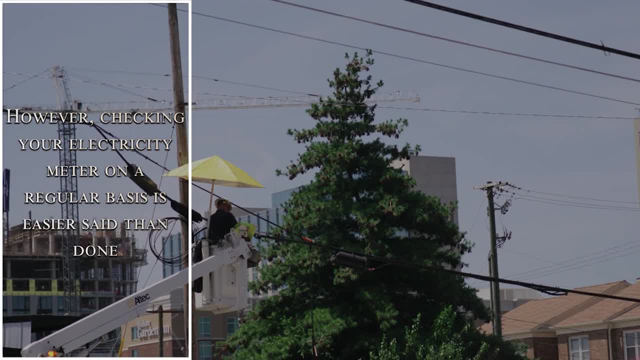 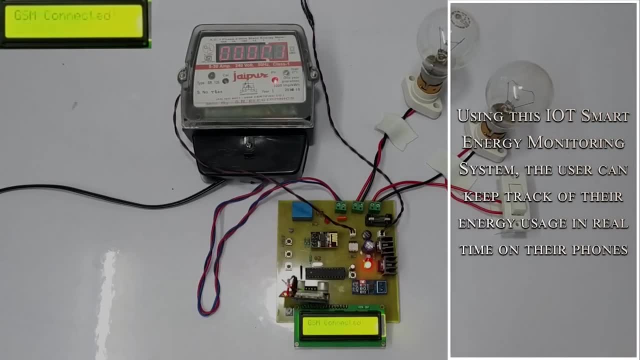 requirements. However, checking your electricity meter on a regular basis is easier said than done. So using this IoT smart energy monitoring system, the user can keep track of their energy uses in real time on their phones. This system is equipped with theft monitoring that alerts the user upon detecting any sort. 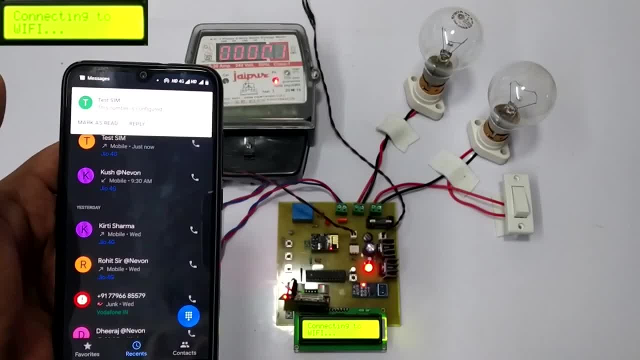 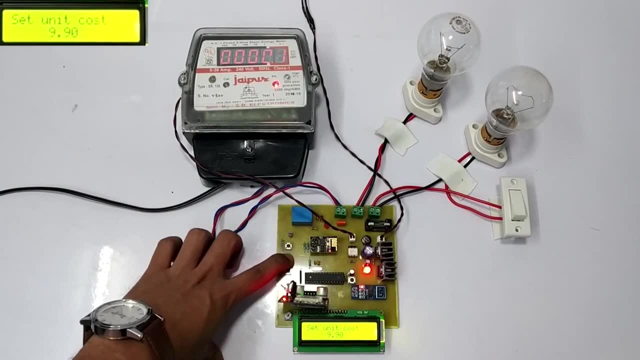 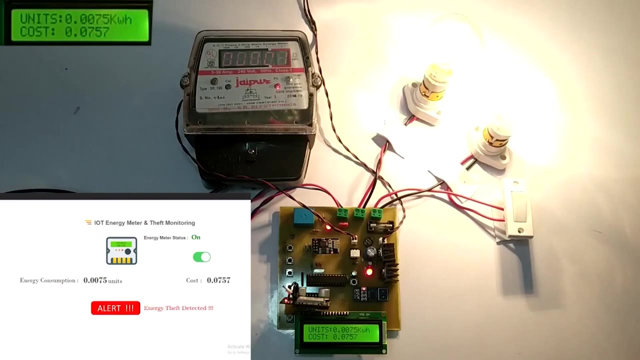 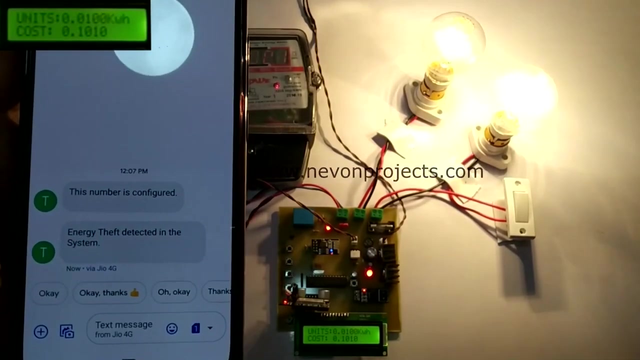 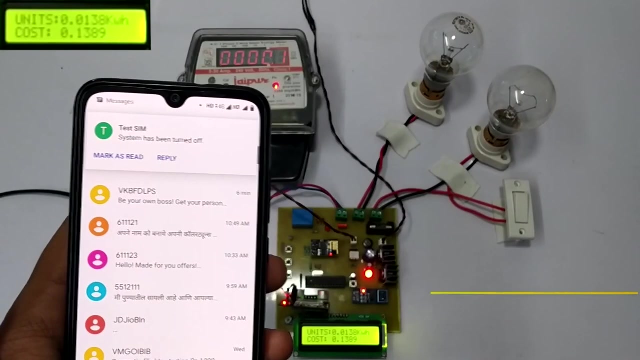 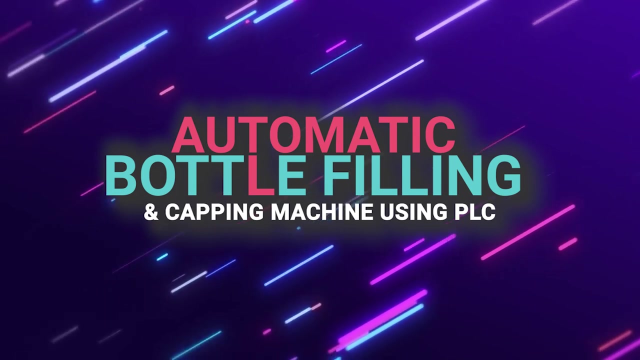 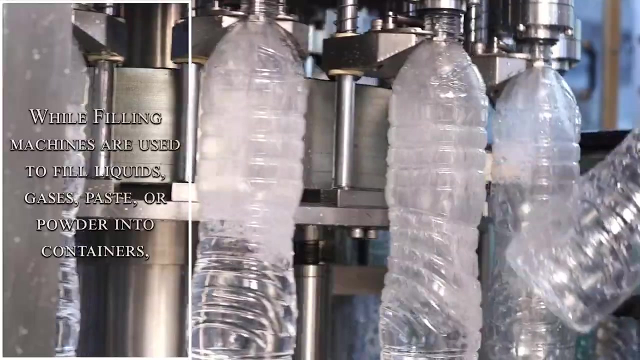 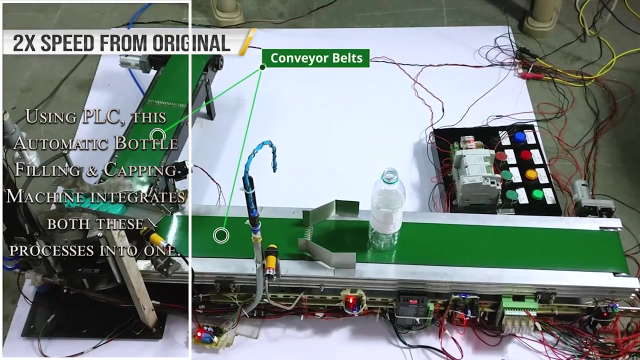 of electricity theft. Automatic Bottle Filling and Capping Machine using PLC. While filling machines are used to fill liquids, gases, paste or powder into containers, capping machines seal the containers after they are filled. Using PLC, this automatic bottle filling and capping machine can also be used to fill the. 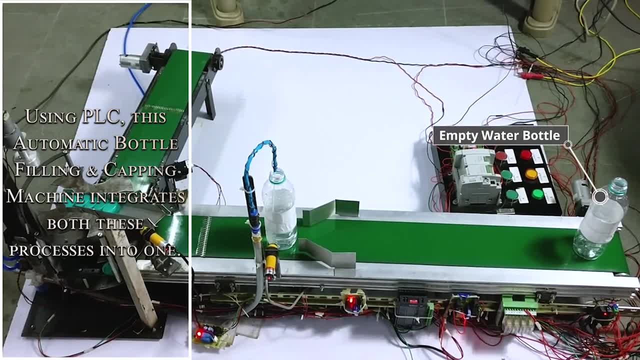 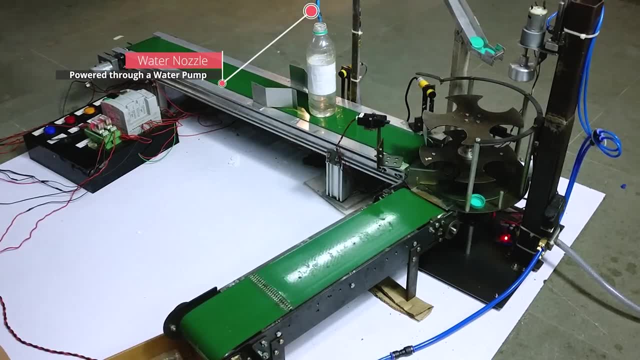 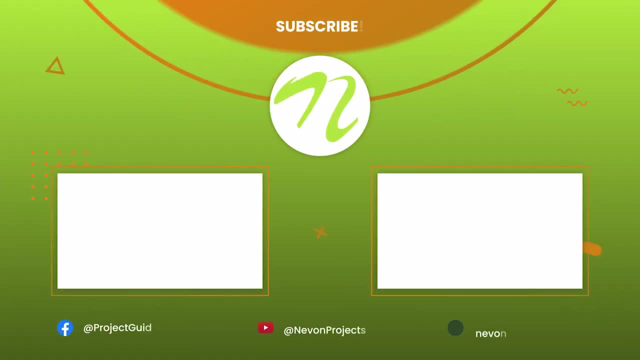 containers after they are filled. The bottle filling and capping machine integrates both these processes into one, The uhh. the Bottle Filling and Capping Machine, integrates both these processes into one.